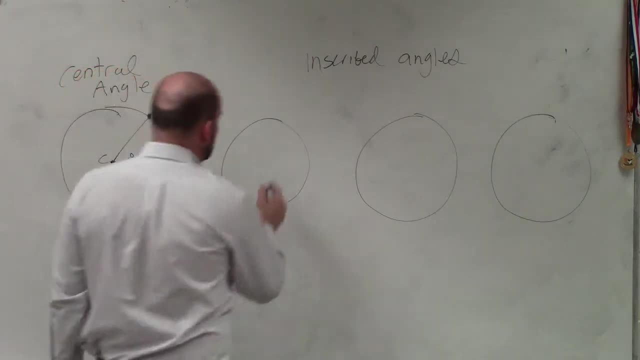 Case 1, case 2, case 3.. Case 1, case 2, case 3.. Now we already talked about an angle that has a vertex at the center, So we're going to have our center, Okay. 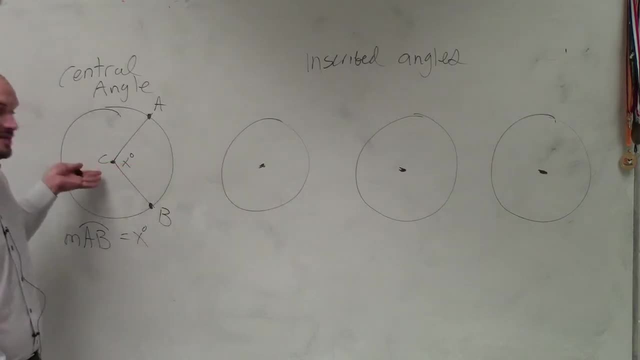 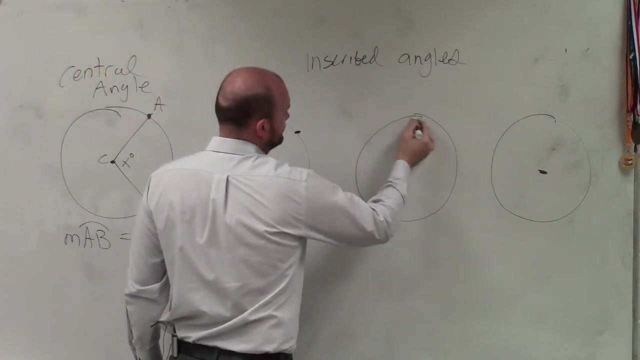 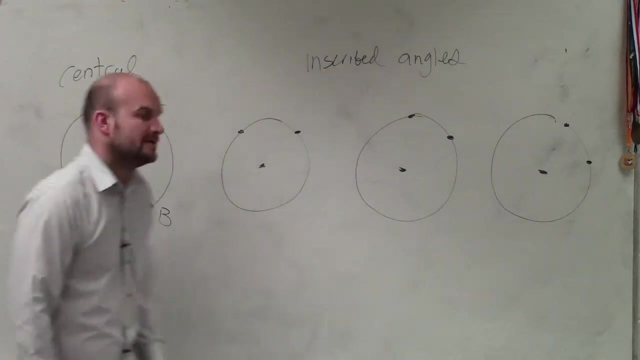 However, our vertex is no longer going to be at the center, like it is for a central angle. Our vertex is now: let's have AB, AB, So case 1, an inscribed angle. All right, And let's call these AB. 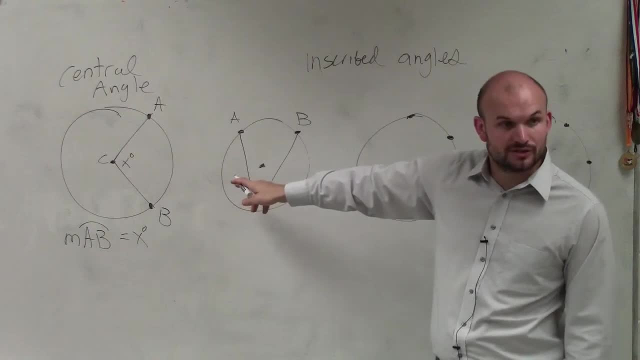 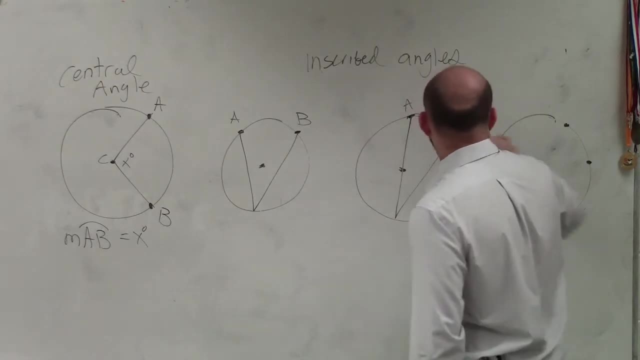 It can either have the center inscribed in between the angle, it can have a line that goes through it, or it can have the center outside of it. Now, what's important about an inscribed angle is that one. you guys notice that the vertex is not. 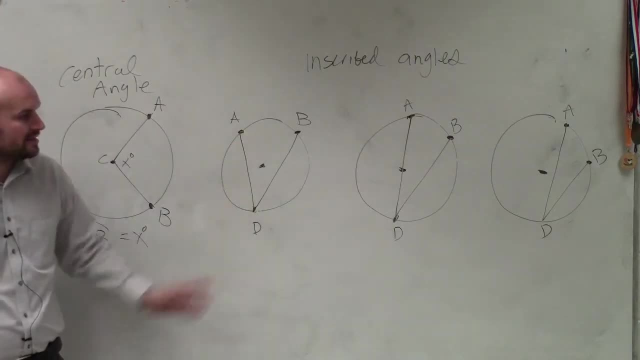 it's not at the center, the vertex is on the circle, All right. And also what's important is, if you guys remember we had the central angle was equal to x. right, It was equal to that angle For an inscribed angle. Layla, the measure of an inscribed angle. 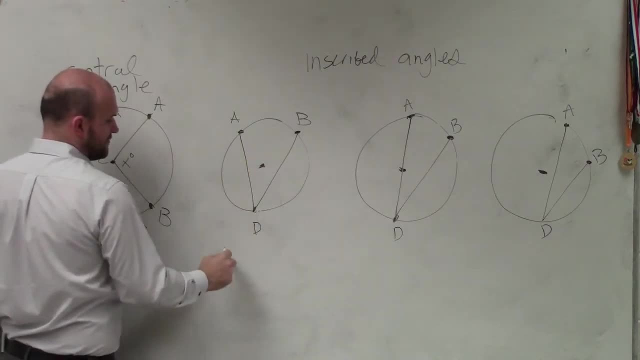 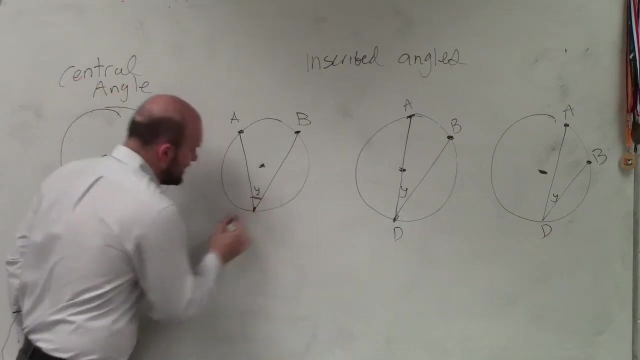 so we'll say measure of angle D. all right, fine, What do you want to call it y? Let's call these all y. So the measure of angle y, this angle, right here, this angle, right here, the measure of angle y. 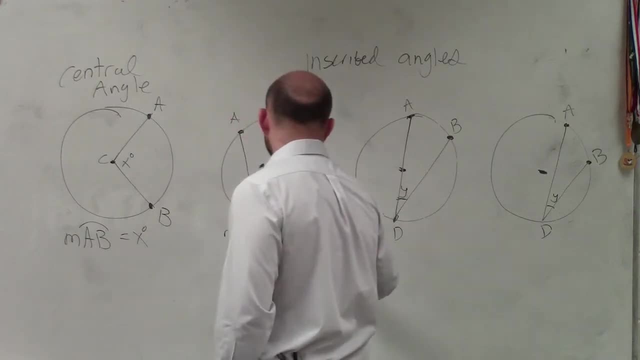 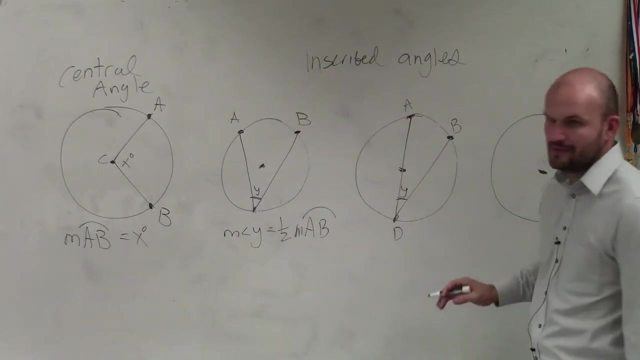 is equal to 1 half the measure of the arc AB, And that's true for all inscribed angles, So I'm not going to write that three times. So again, it's very important: 1 half measure of arc AB. 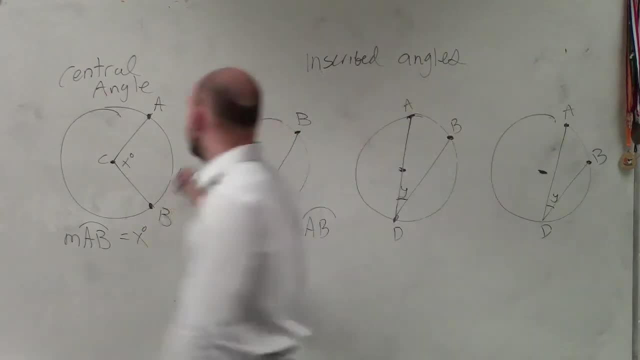 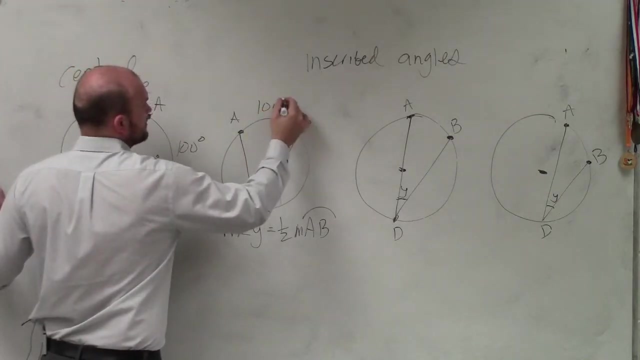 So it's equal to 1 half, 1 half of it. It's not equal to the same. If I said this is 100 degrees, what is this 100 degrees? If I say this is 100 degrees, what is y? 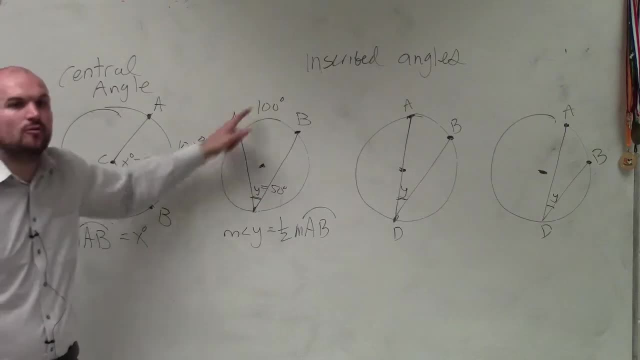 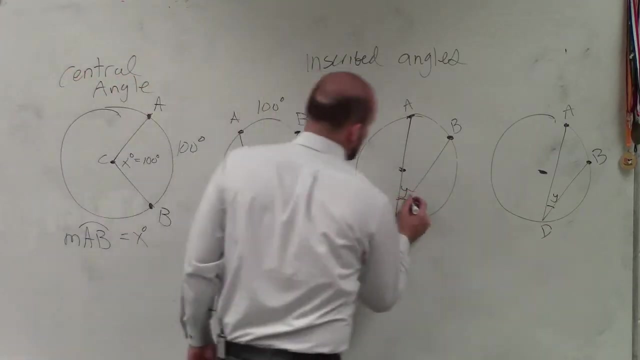 50 degrees The angle is 1 half of what your arc measure is. OK. Does everybody see that? So then, if I say this is 13 degrees, then the arc measure for this one would be Very good. I don't know.